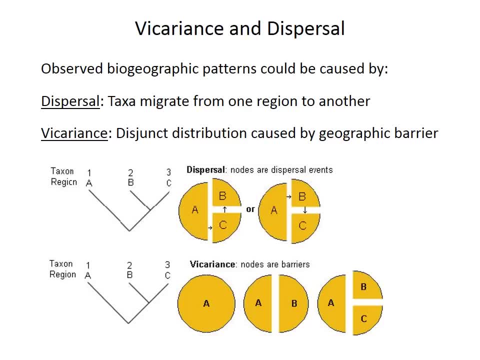 So these disjunct distributions may reflect dispersal, where a new species migrates to an area that's distinctly separated from the area where the ancestral species lived. The top example illustrates that, and it shows how the most primitive taxon, Taxon 1,, the lowest branch on 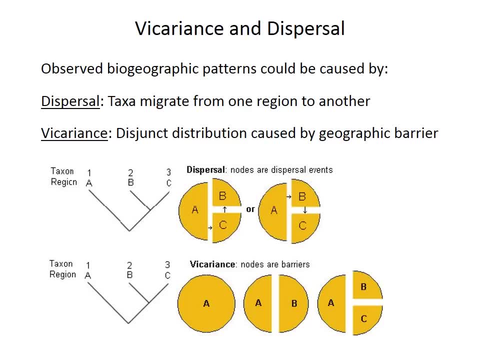 your cladogram inhabited region A, the left wedge of the yellow-orange pi diagram, The more derived species 2 and 3, dispersed to areas B and C. Because we only know that Taxon 2 and 3 share a common ancestor, we can't distinguish between the two different patterns, A to C to B. 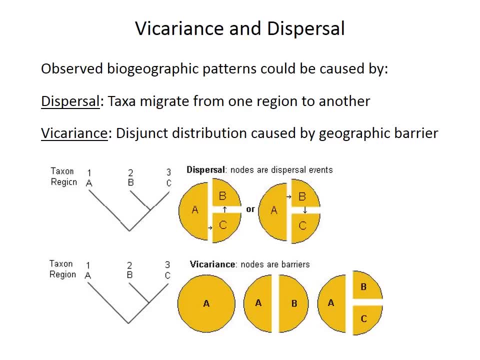 or A to B to C Disjunct distributions may also be caused by, or instead caused by, something called vicarians, In that it's the formation of some kind of barrier, like a mountain range or an ocean basin or a land barrier between oceans, splits a preexisting species into two groups, allowing 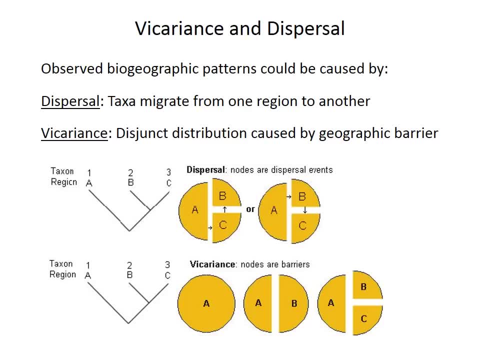 speciation on either side of that barrier. So in the lower example, species one originally lived over the entire circle, region A in the left-hand circle. But that large region was split into two by a barrier And one of those subpopulations in the right-hand wedge evolved into species two in this area. 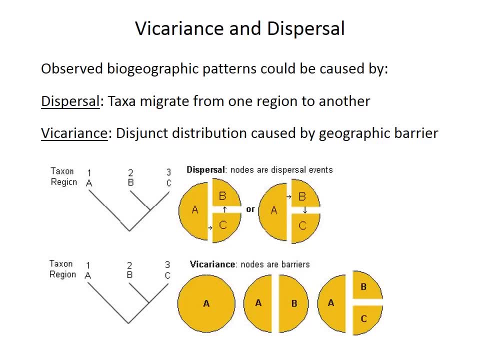 called B Species. two was later split into two smaller groups by another barrier that led to the speciation of taxon three in region C. So in the lower example, species one originally lived over the entire circle, region A in the left-hand circle. 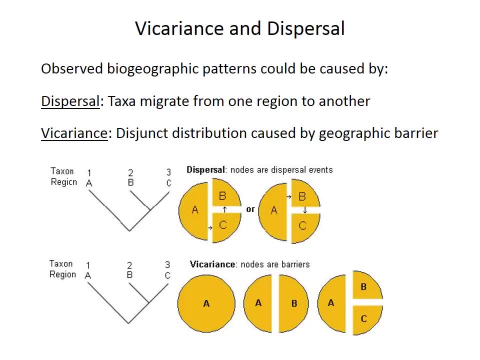 So one thing that you may have noted is that the cladogram and the final distribution- the large wedge of A and the two smaller wedges of B and C- are the same for both dispersal and vicarians, So you clearly need more information to distinguish between these two scenarios. 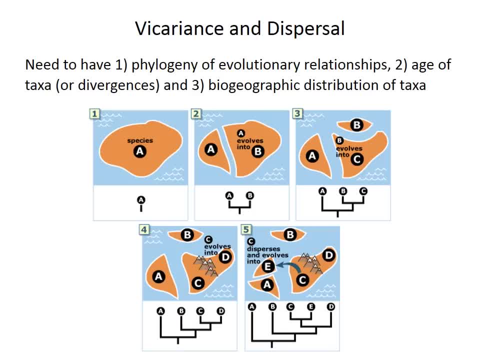 So to test for vicarians or dispersal, to distinguish between those two, you need three things: A phylogeny, Data on the age of the taxa or on the timing of the division, Timing of the divergences, for example, from biocertigraphy. 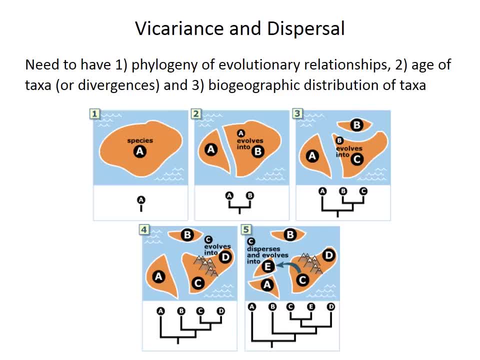 And information about the distribution of the taxa at different time intervals. So the key, critical piece of information that you need is the geographic distribution of the ancestral species. So let's take this example illustrated here: The evolution of species B. the one in panel number two in the figure is an example of 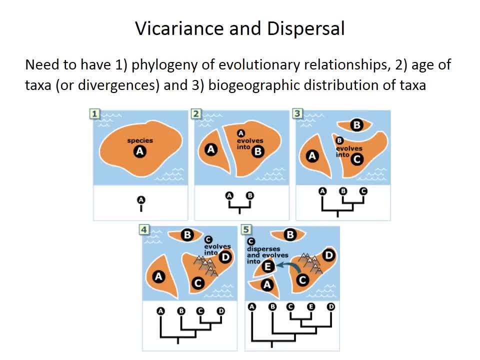 speciation during vicarians, Because species A used to live in the middle of the circle And species B used to live in both areas, including the area in which B is now found. If you looked at the stratigraphic distribution of fossils in that region, you should find. 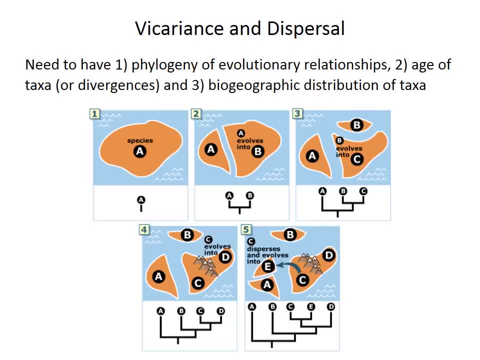 A in older rocks and B in younger rocks. The evolution of species C is also driven by vicarians, because B occurred in both regions in panel three before C evolves in just one of them. The same is true for the evolution of D- Also bicarians. 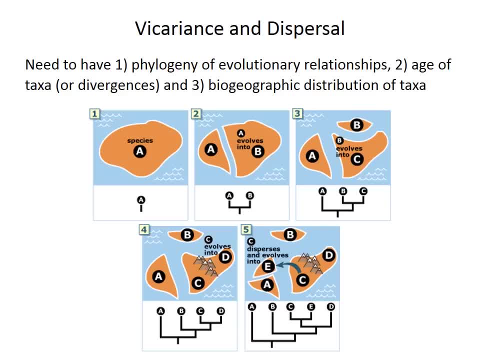 The evolution of species C is also driven by vicarians, because B occurred in both regions in panel three before C evolves in just one of them. The evolution of species E is also driven by vicarians. Vicarians is supported by the former presence of species C in the region now inhabited by. 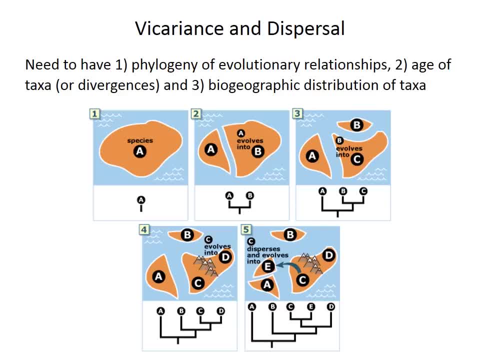 D, But the evolution of species E in panel five is different, however. It's dispersal and not vicarians, because the ancestral species, species C, was not present in the region occupied by the descendant species E. E is found in a new area where C was never present. 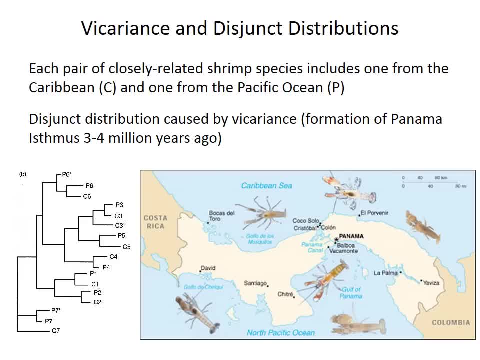 So here's an example that is most likely vicarious from modern organisms. So this study looked at seven species of shrimp from the Pacific coast of Panama. those are labeled P1 through P7 on the cladogram, and seven species from the Caribbean side labeled 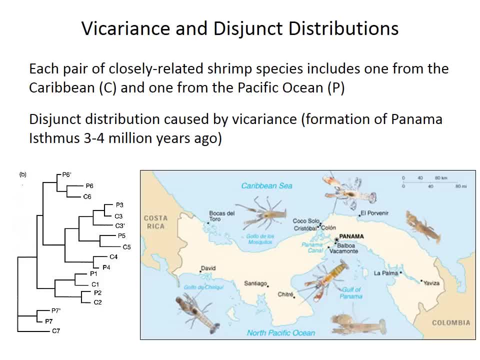 C1 through C7. In all cases on the cladogram the species pair up C1 with C2, C1 with P1,- sorry- P2 with C2, C3 with P3, so forth. So they're called sister species because they are most closely related and they shared a 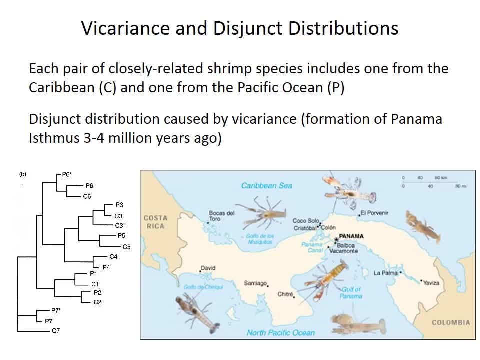 single common ancestor. The disjunct distribution having the closest related species- one on the Caribbean side and one on the Pacific side- is best explained by vicarians after formation of the Panama isthmus around three or four million years ago or so. 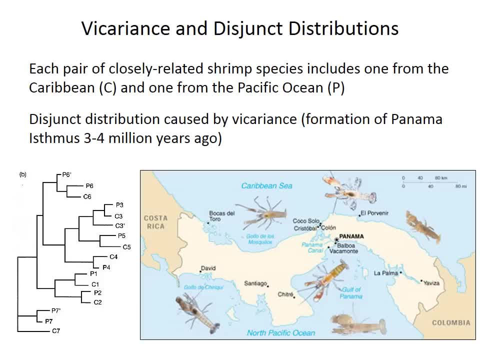 So this study uses DNA, so all the species in the cladogram are living, but the particular prediction that we would make would be that each species pair- C1 and P1,, C2 and P2, evolved from an ancestor that was more widely distributed in the past. 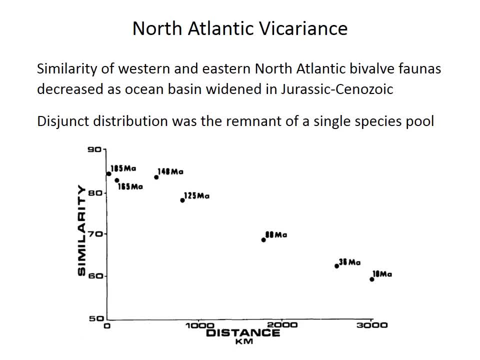 So here's another observation that's most likely vicarious, and people have observed that the similarity of fossil bivalve faunas on the western side and the eastern side of the North Atlantic Ocean decreased from the Jurassic and Cretaceous through the Cenozoic. 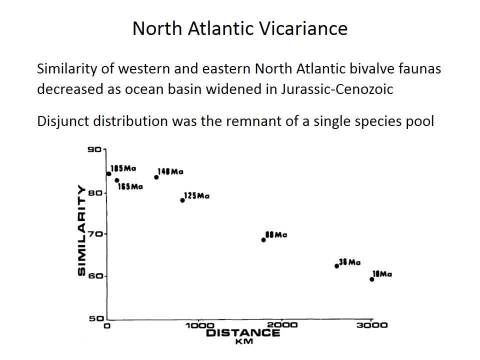 to the present. So early in the spreading of the North Atlantic, say like 185 or 165 million years ago- the two left-hand dots on the graph- the ocean basin was narrow and that means that the larvae of many species could drift from one side to the other. so there was quite a lot. 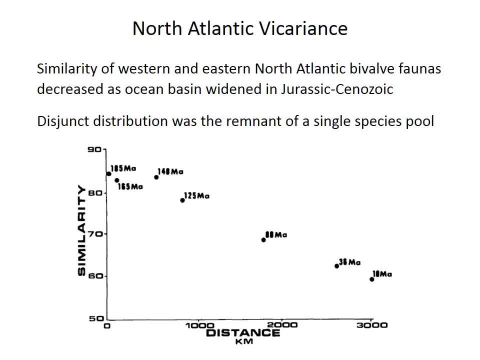 of similarity between the western and the eastern sides, But as the ocean gradually widened, say 125 million years ago or 88 million years ago, progressively fewer species had larvae that could travel across that wide distance and therefore the species composition on each side gradually evolved to be increasingly 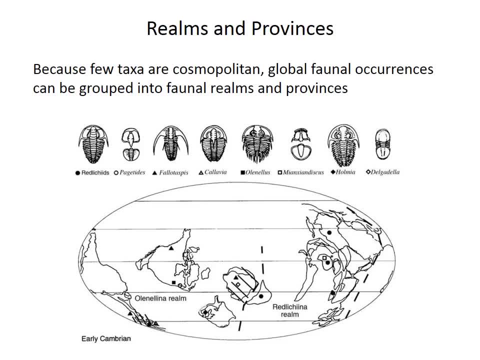 distinct. So, because of larval dispersal limitations and the speciation related to vicarious and dispersal, different parts of the world contain different species. This is a fairly obvious and intuitive fact, But it's not always the case. It provides us with some interesting tools that we can use. 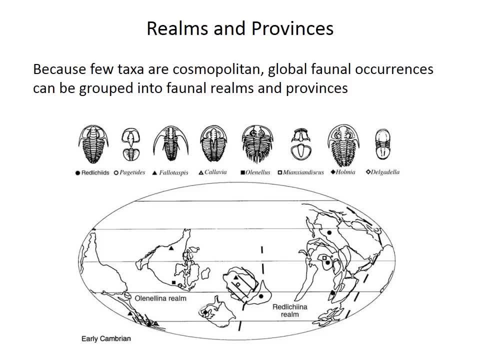 So, as a result, we can divide the globe into biogeographic realms and provinces, or faunal realms and provinces, Like in this Cambrian trilobite example. the paleogeographic map shows that North America and Europe on the left-hand side, in the center, were dominated by trilobites belonging to.